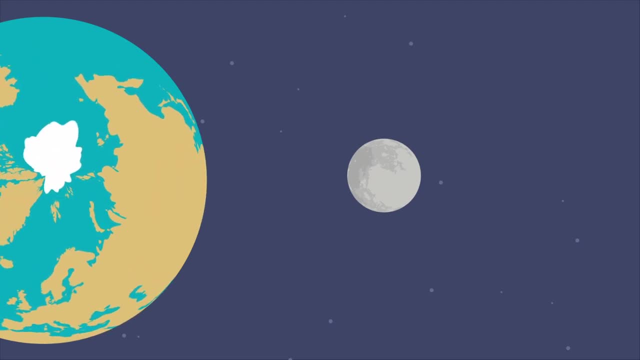 Earth. The moon is a smaller object than Earth, so its force of gravity is weaker, But since the moon is so close, the pull of its gravity is still significant. As the moon's gravity pulls on Earth's water, the water bulges in the direction of the moon. This is due to something. 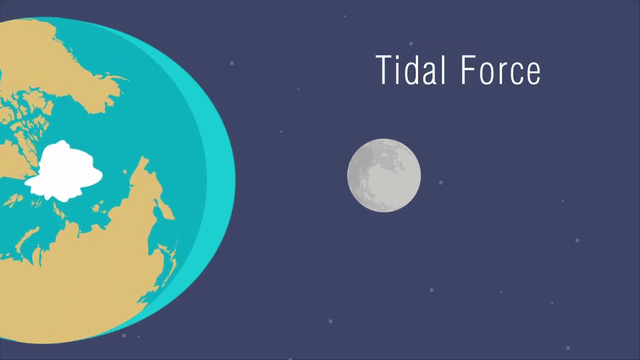 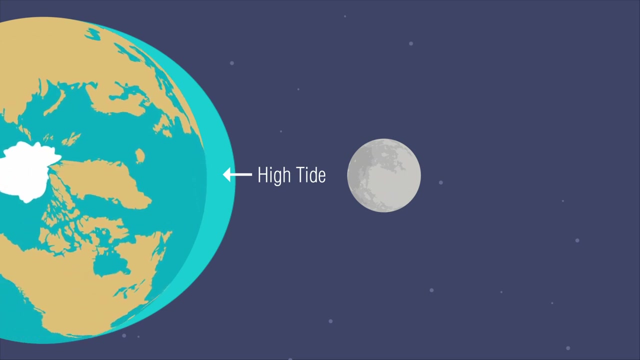 called the tidal force. Because of this tidal force, earth's water on the side of the moon always wants to bulge out toward the moon. This bulge is what we call a high tide, As your part of Earth rotates into tipthe questioningand energy. 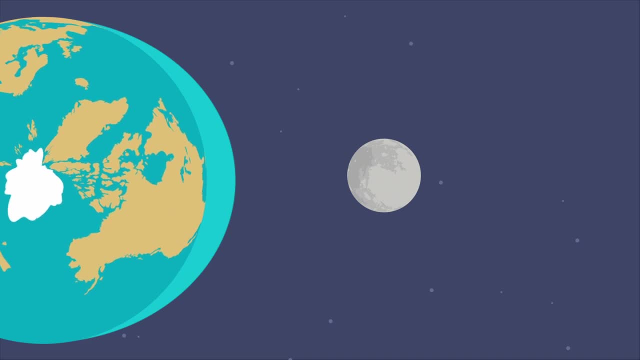 12TUENOW the 1920's, the besch��s of schon time ничего POOLS. OTHER PLANETES that move towards the JSATOבד Woods discuss. water on the side of the moon always wants to bulge out toward the moon. This bulge is what we call a high tide. 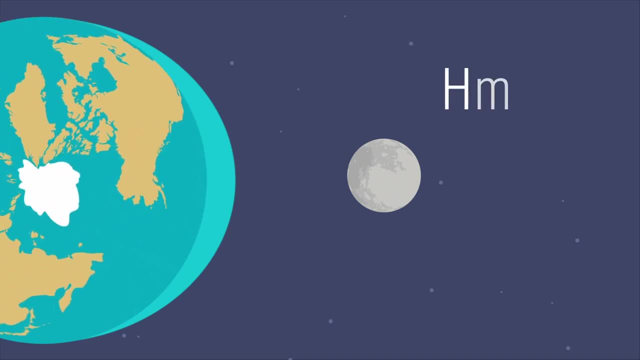 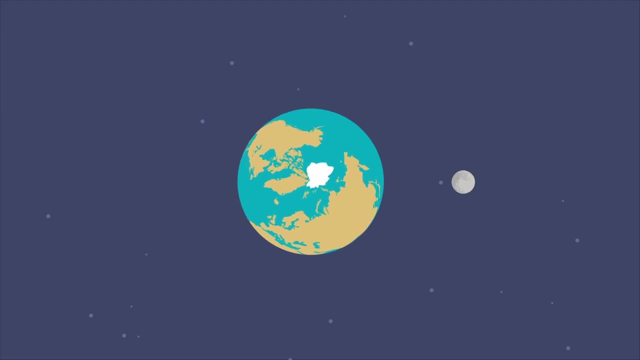 that explains the first high tide each day, but what explains the second high tide? this is where things get a little tricky. as we mentioned earlier, when the moon's gravity pulls on one side of earth, it creates a tidal bulge toward the moon, but the tidal force actually 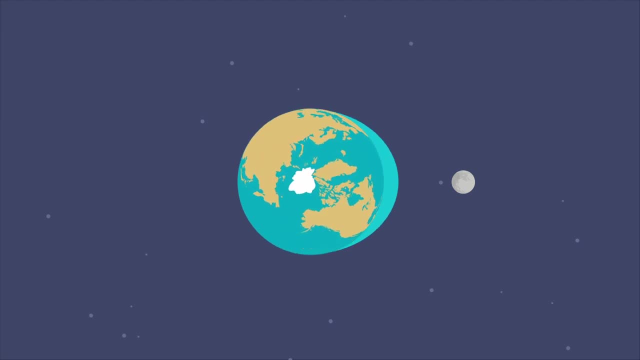 affects the whole planet, not just one side of earth. the total effect of the tidal force is that earth experiences a squeeze which causes the water to bulge on two sides. these two bulges explain why, in one day, there are two high tides. earth's surface rotates through each of the bulges. 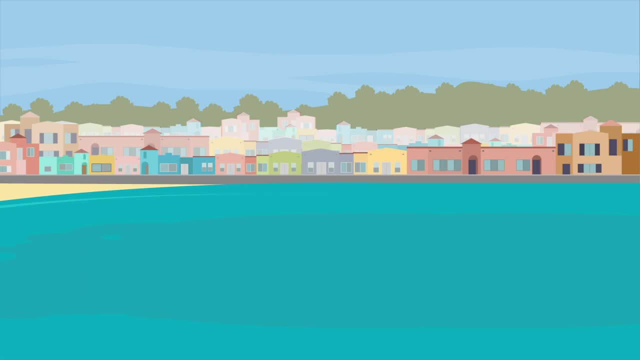 once a day. as earth's climate warms and oceans rise, high tides are becoming higher. sometimes this leads to flooding in communities near the coasts. high tide flooding happens when tides are caught in the middle of the ocean and the tides are accurate in the middle of the ocean. 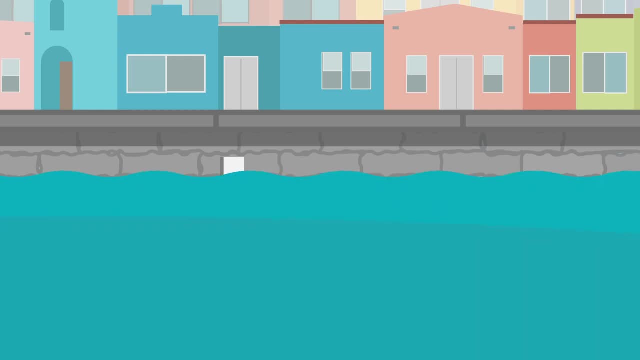 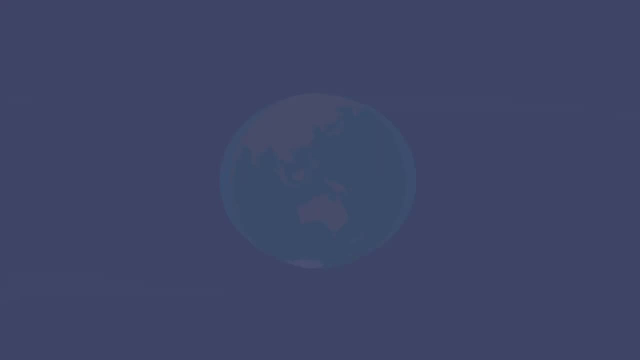 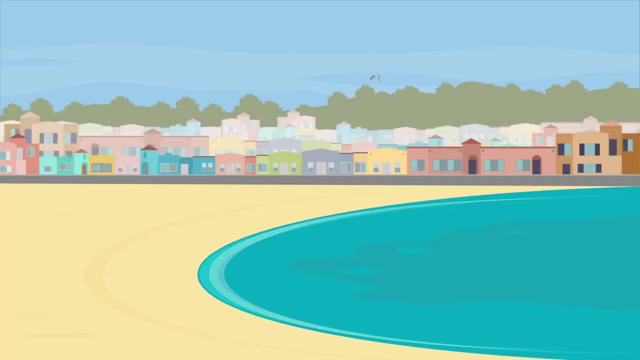 are approximately two feet above the average high tide. this is when ocean water starts spilling onto streets or bubbling up from storm drains. scientists use information from many sources, including noaa's goes r series weather satellites, to study these high tide floods. coastal communities can use this information to better plan for the effects of rising tides in the future.